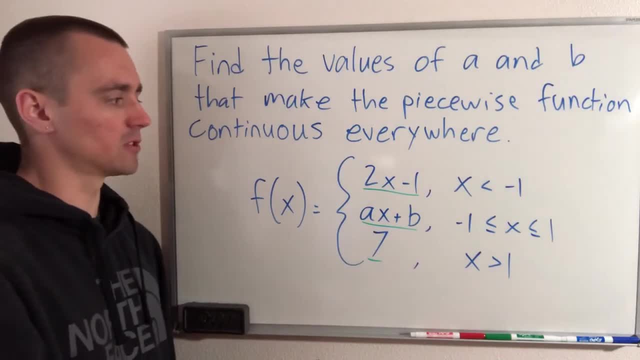 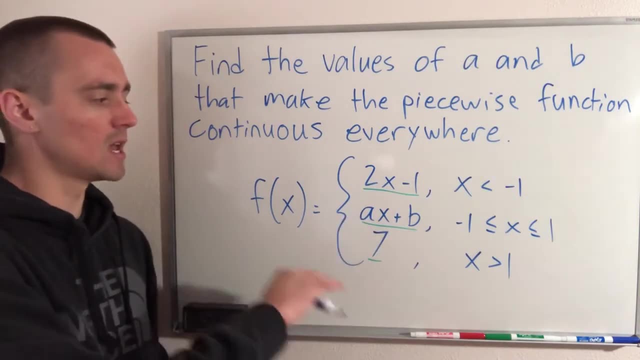 that each of them would be continuous by itself. So if we just looked at, the function y equals 2x minus 1, or the function y equals ax plus b, or the function y equals 7,, any of those three functions would be continuous for all x. 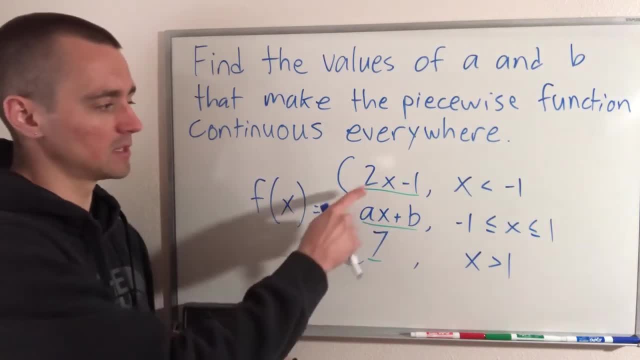 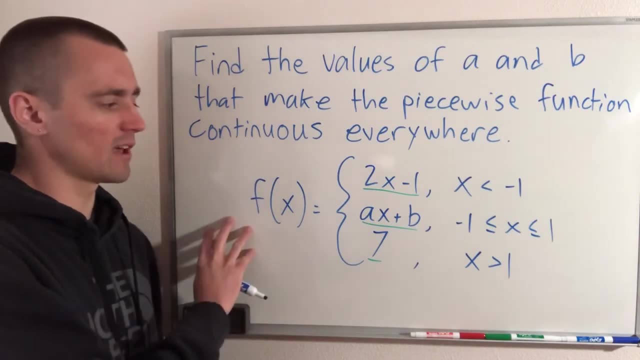 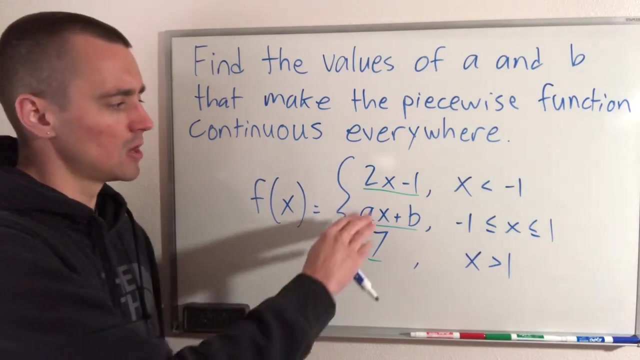 values, No matter what a and b are, because they're all just linear functions which are continuous everywhere for all x values. So what that tells us is: when we have a piecewise function that's made up of three individual pieces, that would normally be continuous everywhere by themselves. we just need to make sure. 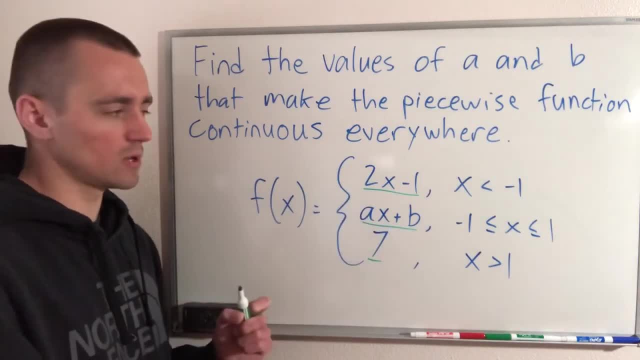 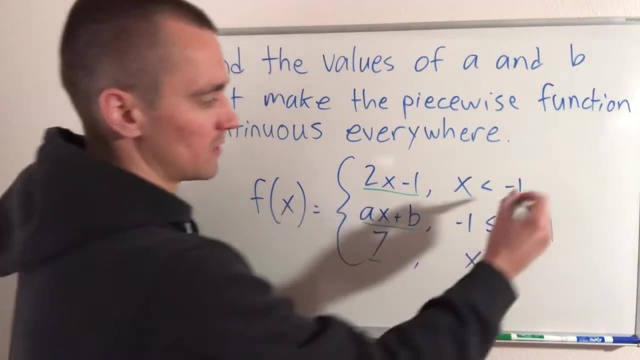 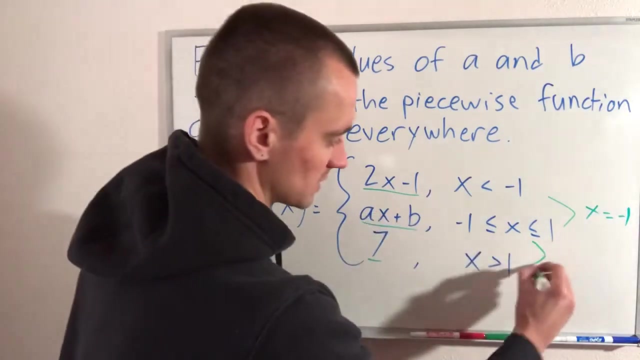 that our piecewise function doesn't have a jump discontinuity when we switch from one function to the next. So in other words, we want to look at when we switch this function to this function that happens at x equals negative 1.. And then again we'll switch from this function to this function when x equals 1.. 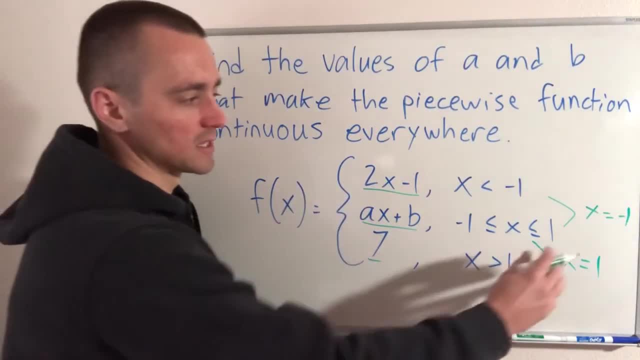 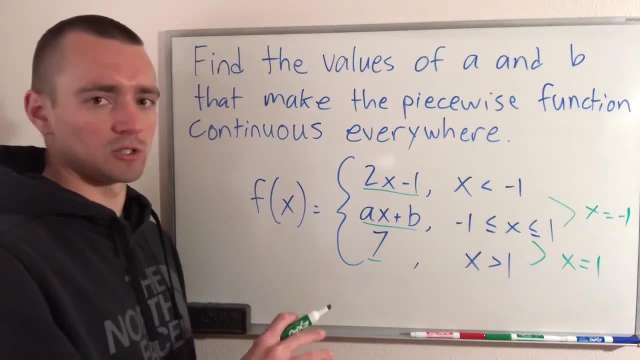 So all we really need to check is that our piecewise function is continuous: at x equals negative 1 and at x equals 1.. And if we can do that, that a and b combination would make this function continuous everywhere. So all we have to do 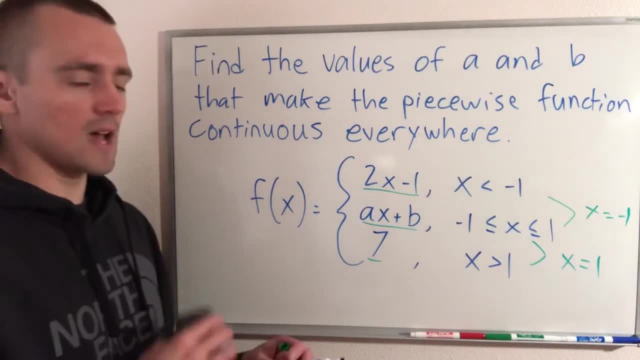 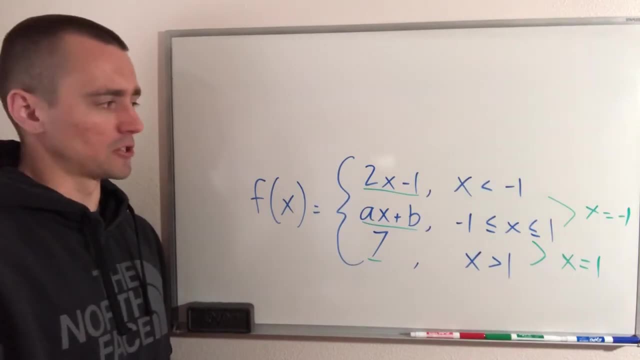 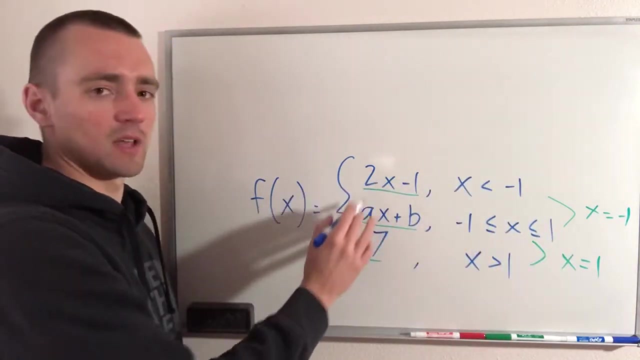 to do that is consider the height of each of these functions at these couple of points, And what I mean by height is the output of those functions. So, in other words, when we have our input, is x equals negative 1, we need to make sure that these two functions have the same output so that they line up when we switch between them. 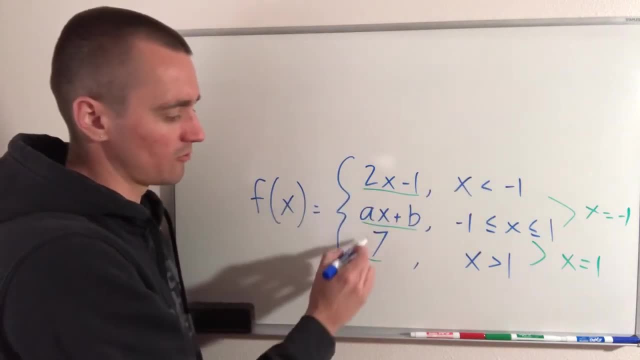 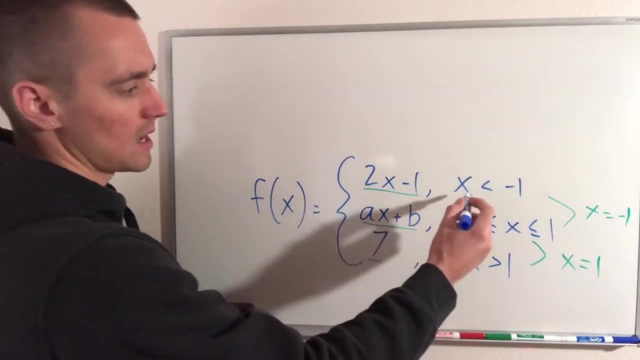 at negative 1.. And then again we need to make sure that these two functions have the same output when we switch between them at x equals 1.. So all that means is we will take x equals negative 1 and we'll plug that into these two functions and set them equal to make sure. 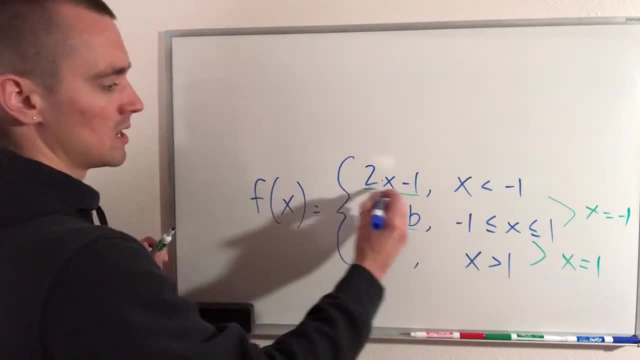 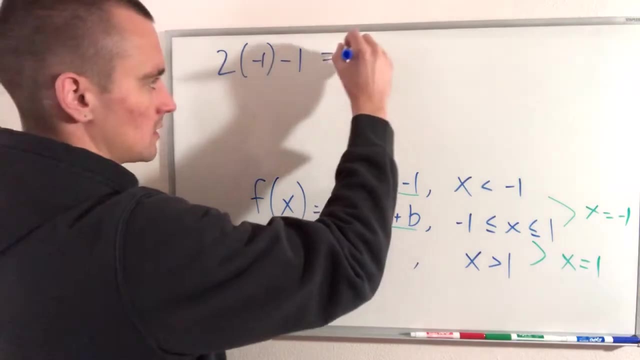 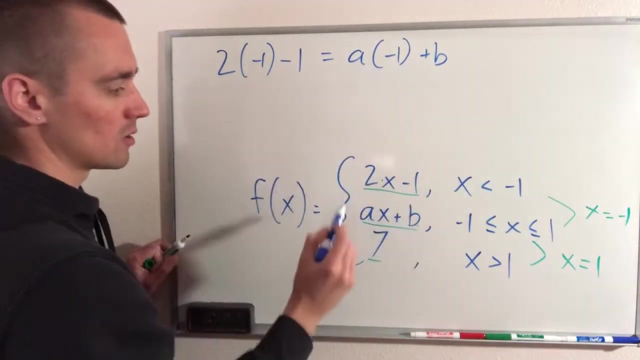 they have the same output. So when x equals negative 1, this function will give us 2 times negative 1 minus 1.. And this function will give us a times negative 1 plus b. So this is the output of this function when x is negative 1.. And this is the output of this function. 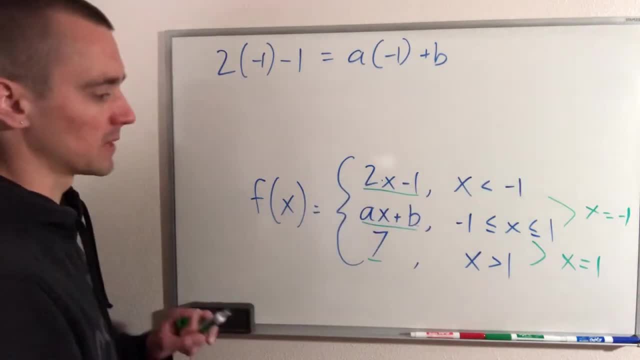 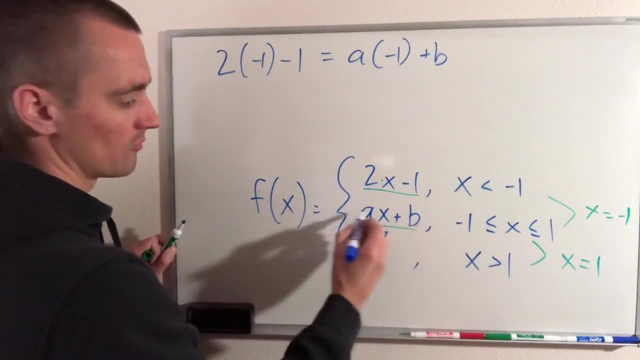 when x is negative 1.. So then, the other thing we need to make sure is that this function has the same output as this one when x equals 1.. So when x equals 1, the output of this middle function here will be a times 1. 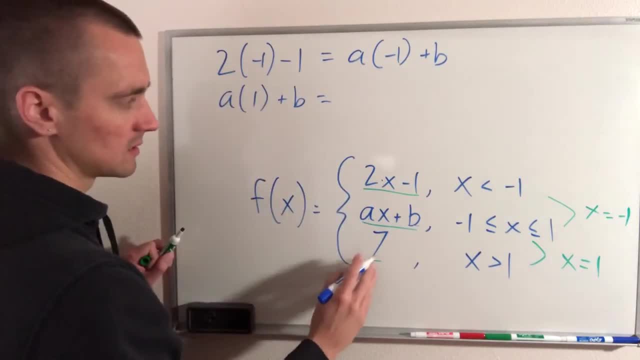 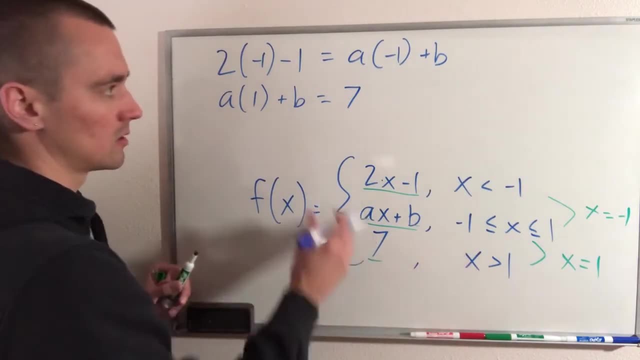 plus b, And that needs to have the same output as 7.. 7 is just a constant. The output of this will always be 7 for any x value. So when x is 1, the output of this function is just 7.. So we need to make sure that our 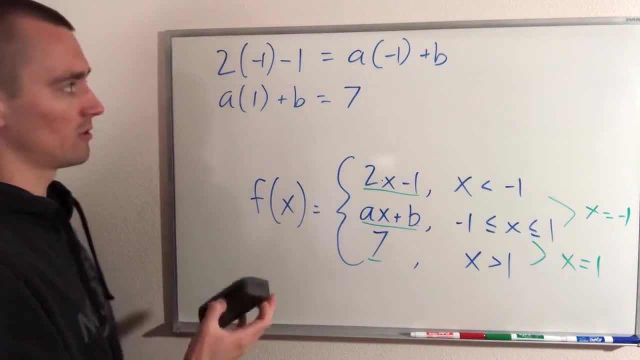 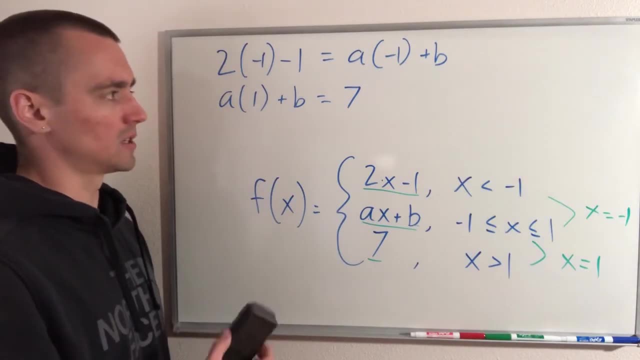 a and b satisfy both of these equations. So all we really have here now is just a system of equations with two variables and two equations which we can solve using a couple different methods. But first thing that's usually easiest to do is start by simplifying these two functions. So let's do that first. 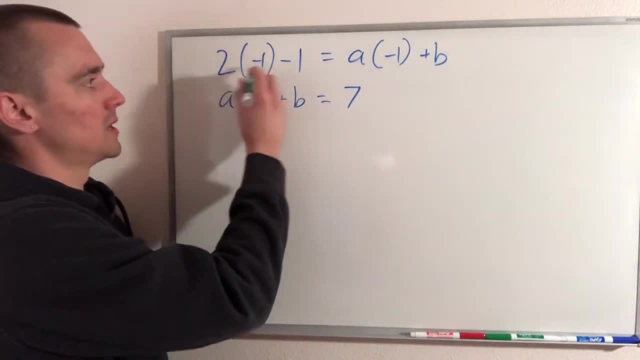 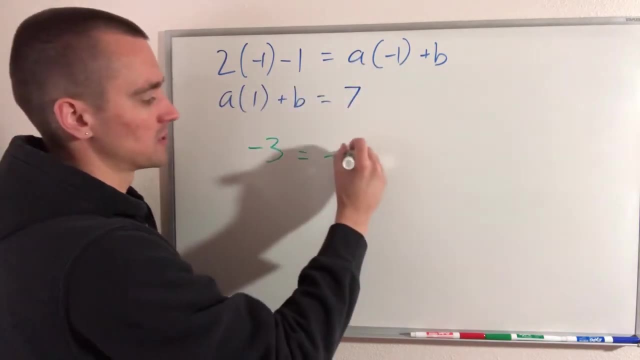 So this first function: here: 2 times negative 1 would be negative, 2 minus 1 would be negative 3. And then this function: here we would just have negative 1 times: a is just negative, a plus b. Then our second function: 1 times. 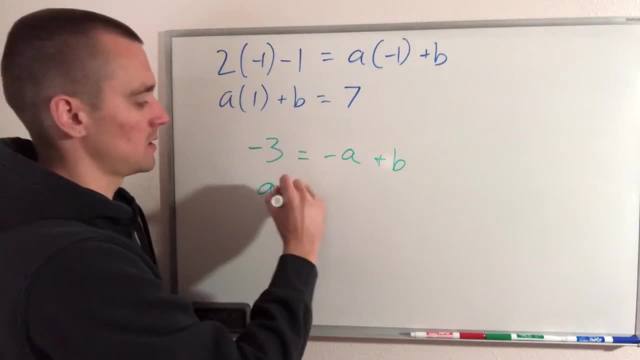 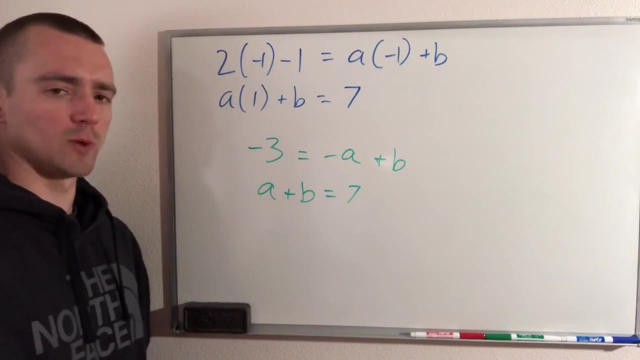 a is just a plus b equals 7.. So now we have these two equations. There's a couple different ways we can solve a system of equations like this. What I'm going to do is use the substitution method, So all that means is we're going to solve one of our equations for one of the variables. 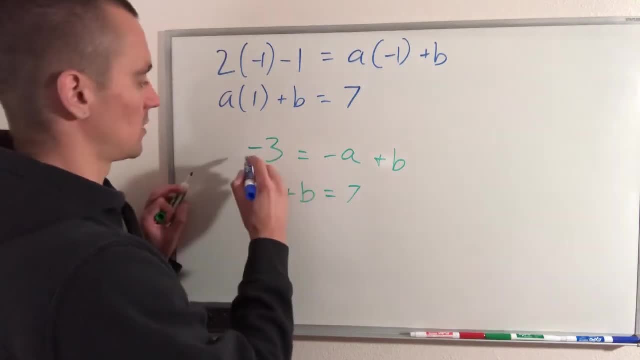 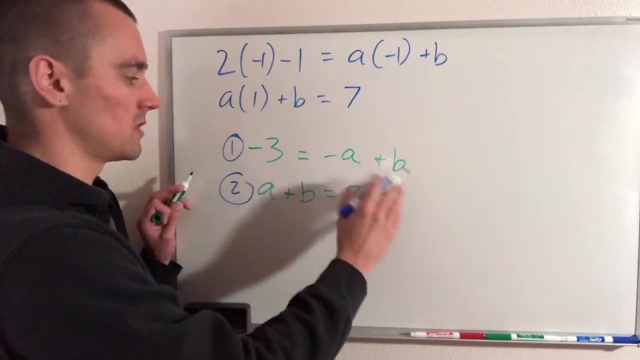 and then plug that into the other one. So let's just take this first equation here And we'll solve this first equation for b, And then we'll take that b value and put it into our other equation. So to do that, all we have to do is 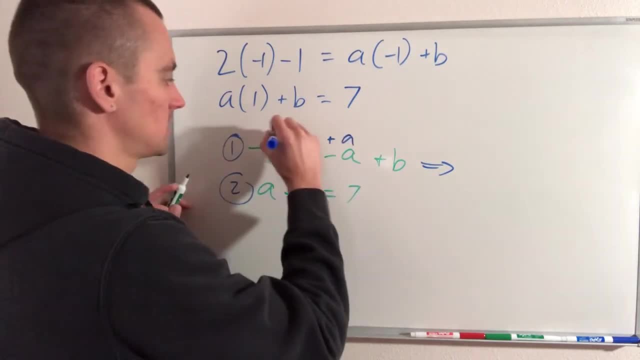 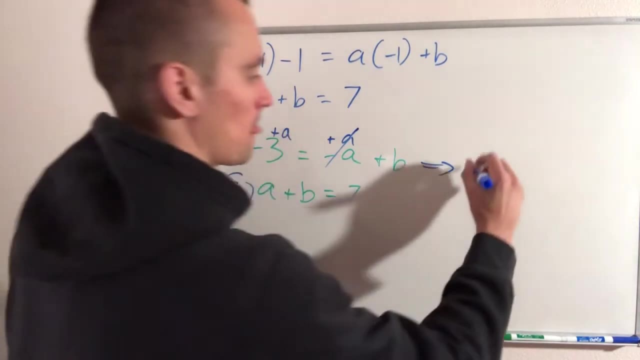 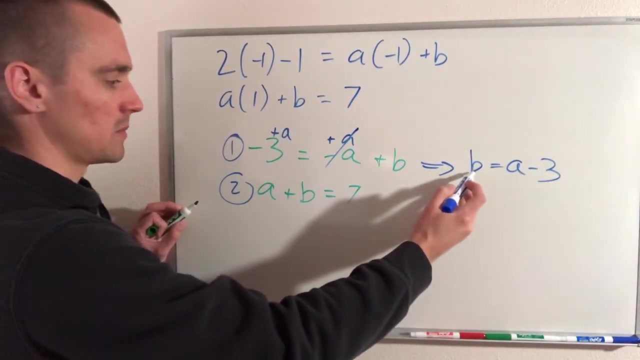 add a over to this side. So we'll add a to both sides and we will get those canceling. So we'll just get b equals a minus 3.. So now we know that a minus 3 is the same as b, So we can take this and plug it in for b. 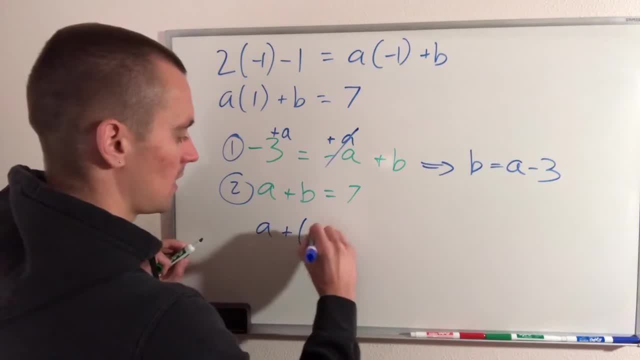 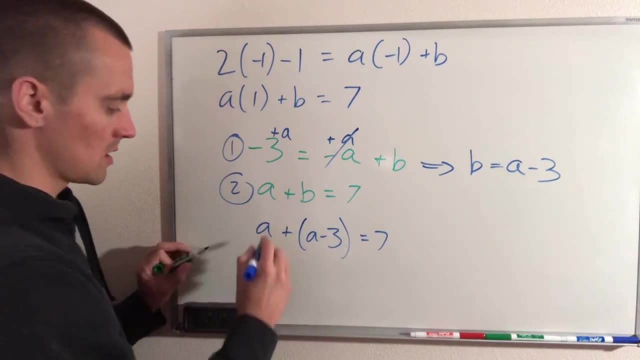 here. So that'll give us a plus a minus 3.. equals 7. Because b and a minus 3 are equal. Now we can just solve this for a, So we'll have a plus a minus 3, equals 7.. 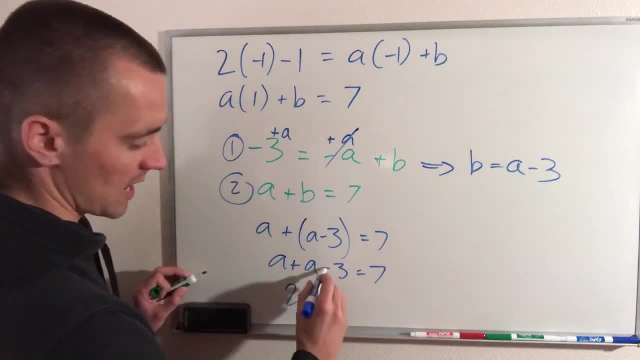 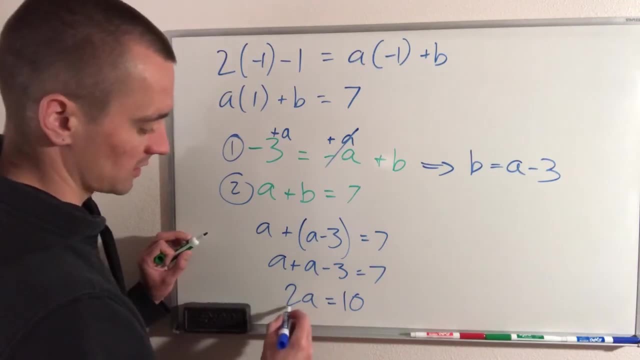 These will just combine to give us 2a, And then if we add our 3 over to the other side, we'll just get 10.. So that tells us a is 5.. Right, Because if we divide both sides by 2, we'll get 2 canceling there.